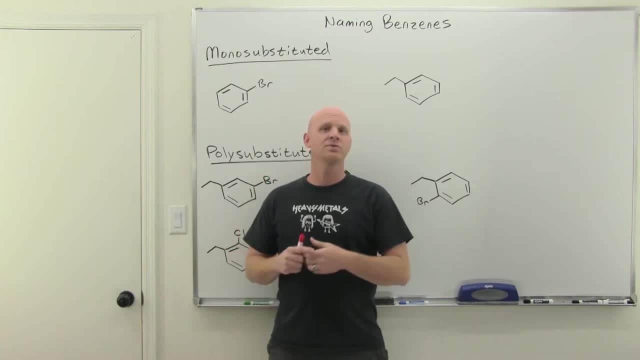 chapters and I will do the same. In this first one we will name benzenes, we'll talk about properties of benzenes and some conceptual understanding associated with them, and we'll identify aromatic compounds. And then in the second chapter, we'll go through and talk about 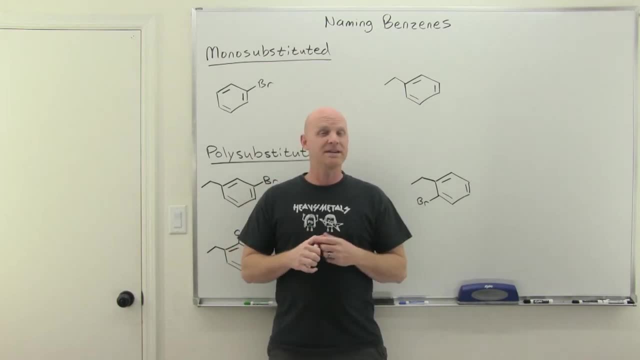 the reactions of aromatic compounds. Now in this lesson we're going to be naming benzenes. We'll name monosubstituted benzenes and disubstituted benzenes and, even more, substituted polysubstituted benzenes. We'll talk about benzenes with special names. We will cover everything you are likely. 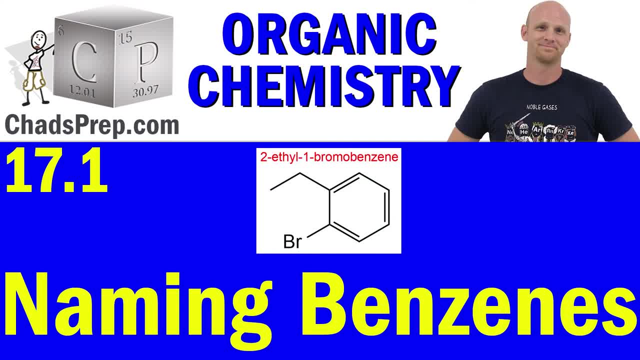 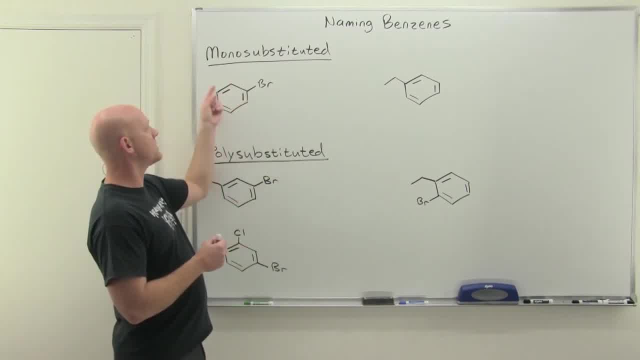 to encounter in your undergraduate class. All right, so just real quick. this little six-membered ring here, which looks like it has alternating single and double bonds, is benzene. It actually doesn't have alternating single and double bonds. There's actually delocalized electrons all the way. 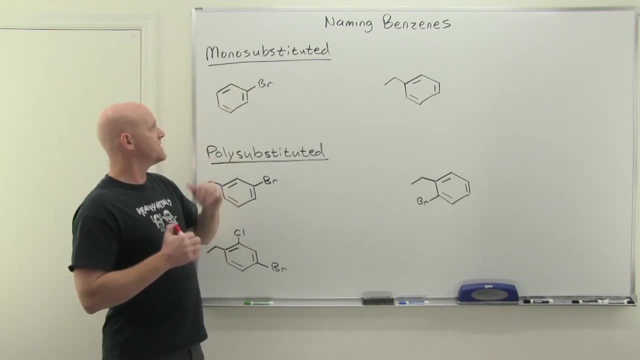 around. This is one of the resonance structures, So just one thing to keep in mind. So we'll start with naming monosubstituted benzenes when you have a substituent coming off there and it'll be very reminiscent to what we saw with cyclohexanes and substituents coming off. So when you name a 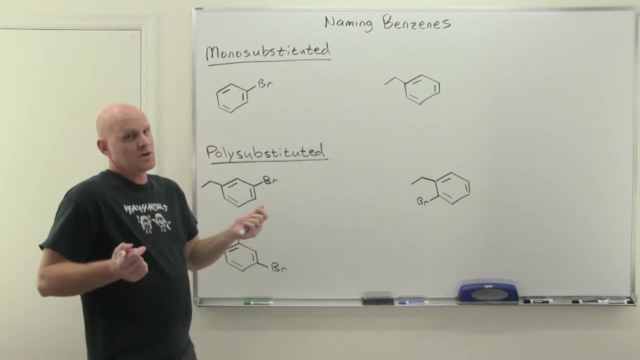 monosubstituted benzene ring here. so your substituent- there's only one- has to be at carbon one That will actually define where carbon one is on your benzene, with six carbons total, And because it's the only substituent. 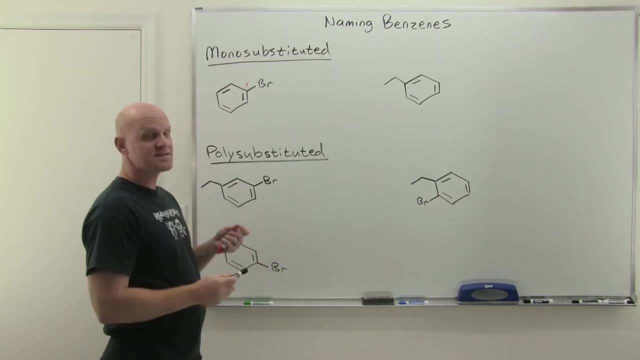 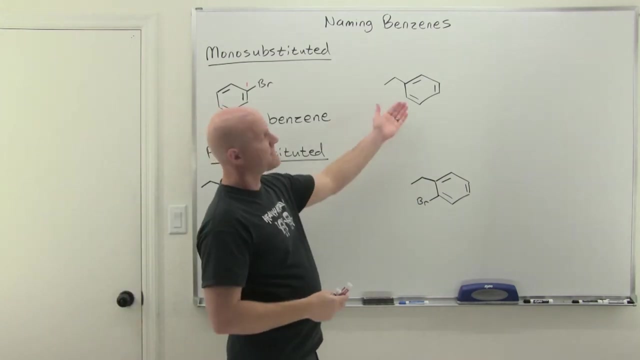 it has to be at carbon one. It is not included in the name. So in this case, instead of saying one bromo and then benzene as the parent chain, we're just going to say bromo, benzene, Cool, There we go. Same thing over here Now, instead of having a bromo as our substituent. 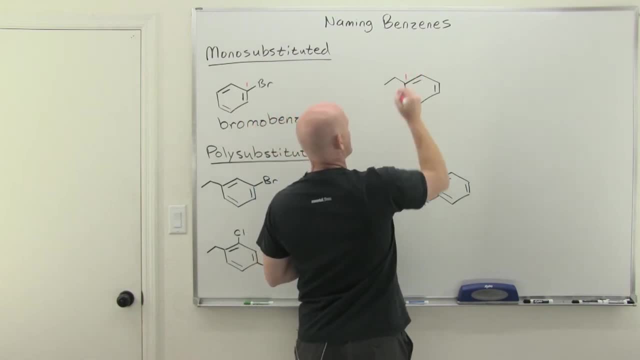 we now have an ethyl group as a substituent, but it's still attached to carbon, number one of the benzene. And then, once again, we don't have to say one ethyl benzene. In fact, we don't say one ethyl. 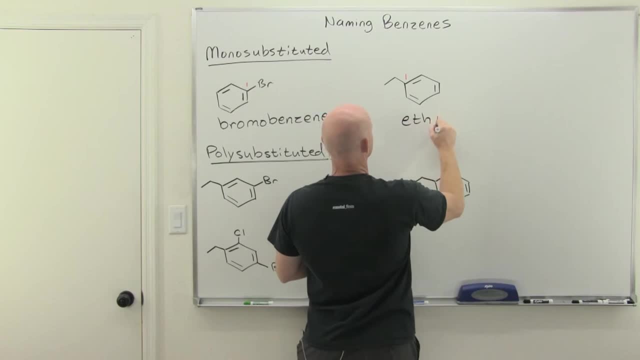 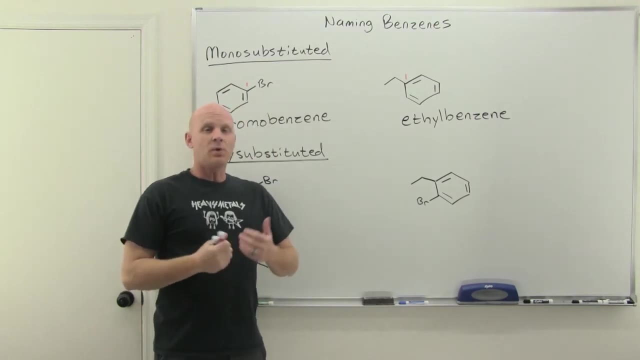 benzene. We just say ethyl benzene, One big word, Cool. So that's monosubstituted benzene. It gets a little more complex with disubstituted benzene and even more substituted. So we're going to do some polysubstituted We'll. 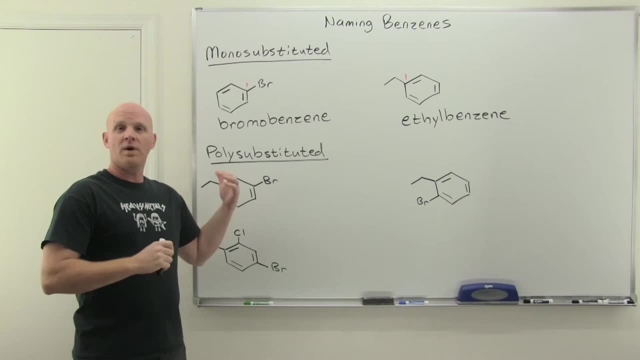 start off with disubstituted ones here. And if you're wondering where's the orthometapara stuff, in case you've already seen that in your course, that's coming. We're going to cover that in the next section here, But we'll kind of use the numerical version here And when we get to some 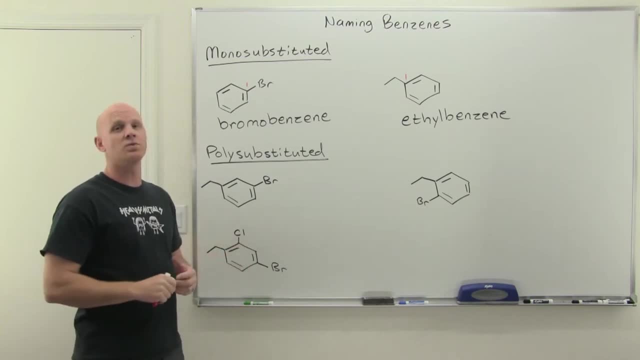 benzenes with special names. in the very next little section of this particular lesson we'll start seeing those orthometaparas. If you're wondering where are those, They're coming. All right. So if we look here, when you've got two substituents with exactly. 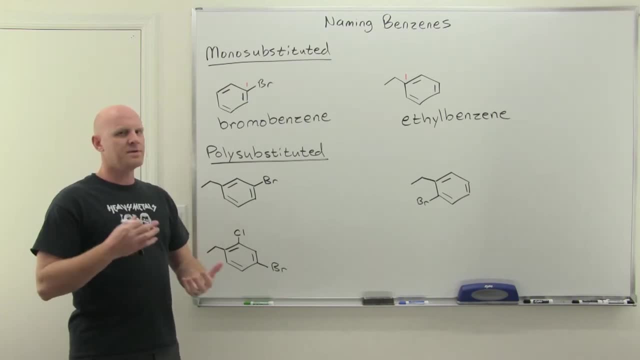 two, just like we saw with cyclohexanes. one of them gets to be attached to carbon number one of the benzene- and the other one's going to get the other number And it's a numerical tie either way. So, like in this case, we have a bromine and an ethyl group and it could be one and three, or 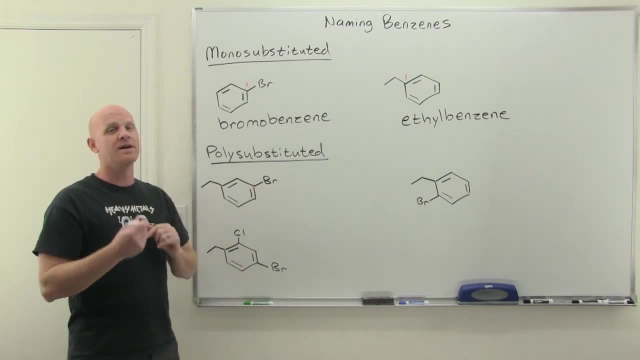 one and three. And since it's an absolute numerical tie, no matter which way you number it, the alphabet breaks the tie on a disubstituted And then in this case bromo comes before ethyl, So we'll number him as number one, And then we number it clockwise or counterclockwise. 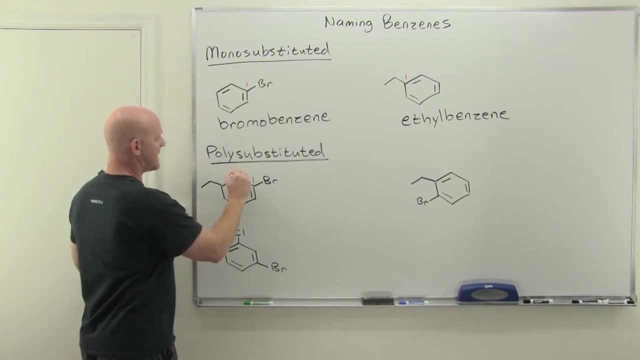 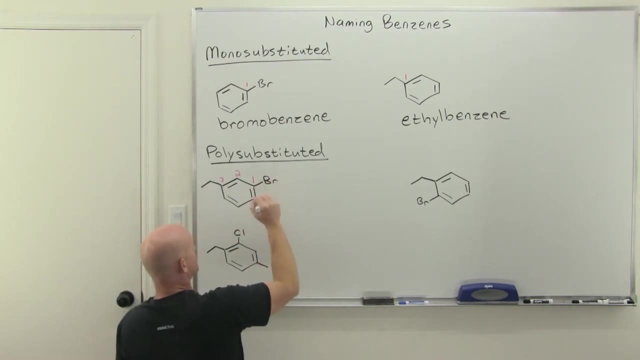 whichever way gets to the second substituent faster. So in this case we'll go counterclockwise. We've got that guy right there, And so we go to name this. You name it in alphabetical order as well, which is still going to follow the same order. So we're going to have one bromo, three ethyl. 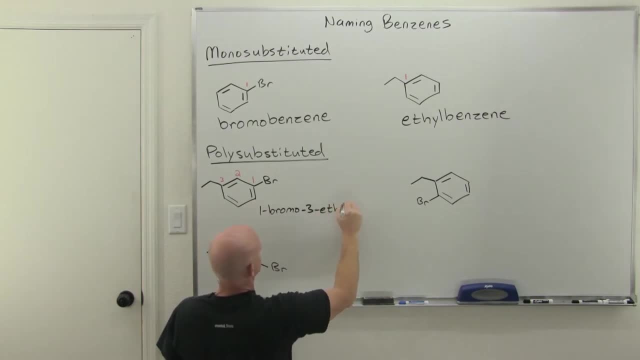 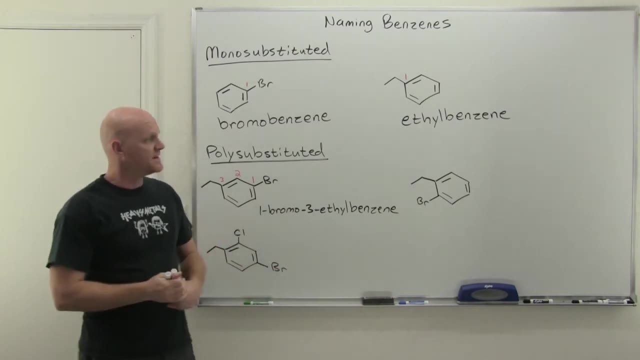 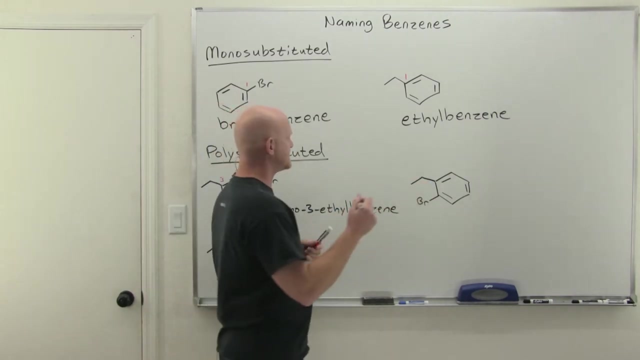 benzene, All right. So same thing with the analogous one over here. So a little bit different numbering, but once again you could have one and two, or one and two, And with a numerical tie. again the alphabet breaks the tie and bromo is going to break it here again. 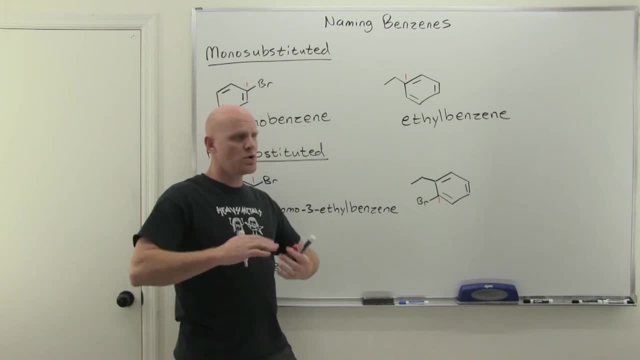 The big thing I want to demonstrate here is that now we're going to count around clockwise. So there's no rule that says you have to count around any direction. It's just whatever's going to give you your second substituent, the lower number, And so we'll number it clockwise. 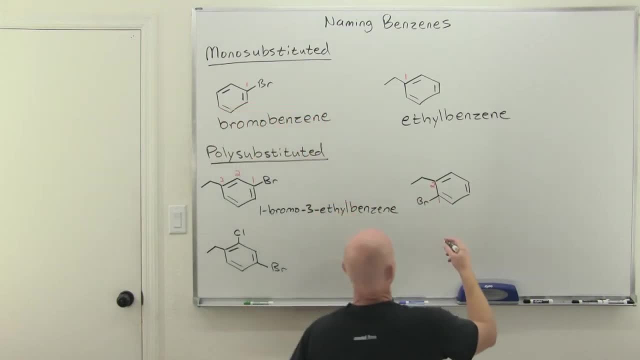 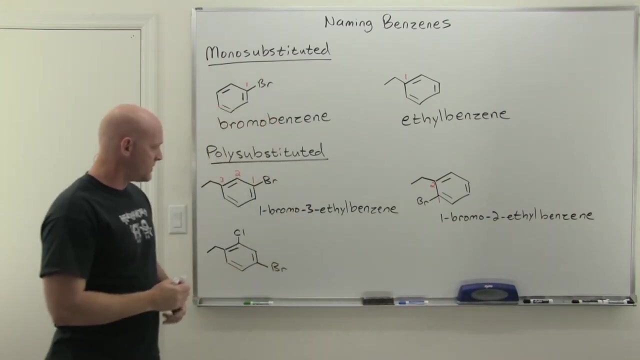 Go around clockwise this time. So, but still naming it, we'll go with the bromo first, And so one bromo, two ethyl benzene, All right. So what if we've got like a tri-substitute or something more substituent? 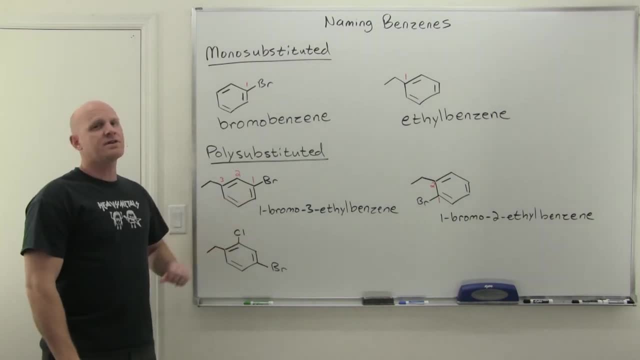 than this, So this gets a little more complicated, but usually this doesn't come down to alphabet breaking the tie, And students often forget that there's not a numerical equivalent, no matter how you number it, And so they often try to do the alphabet breaks the tie on something like this: 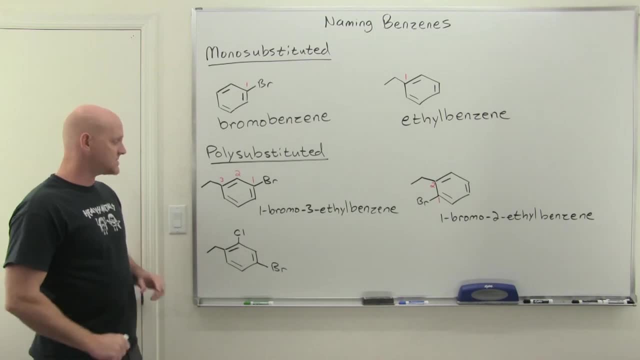 just like with cyclohexanes. But keep in mind that may not actually be the case. A lot of students want to make, where the bromo is here, number one, because bromo comes before chloro and ethyl in the alphabet, But in this case actually it's going to be the ethyl that gets. 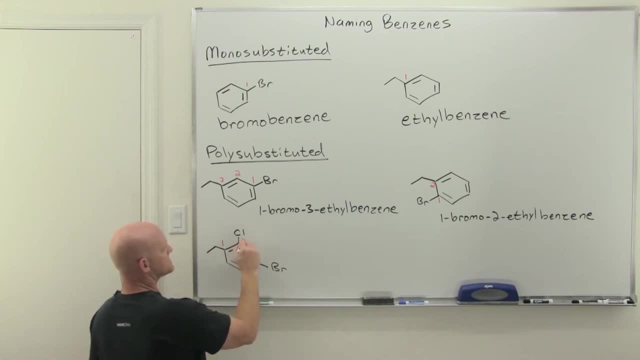 to be number one, because we make him number one, then we have another substituent at two and another substituent at four, And that would be one, two and four. If you make the bromo number one, it would be one and then three. 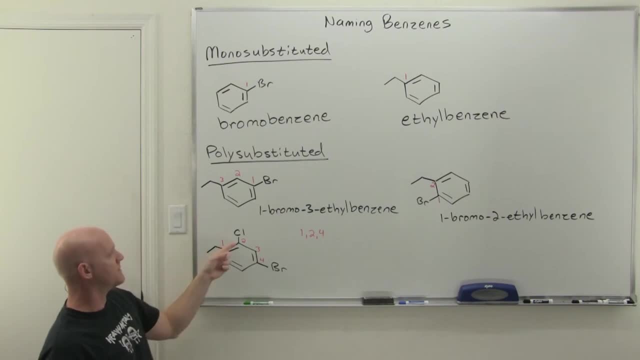 And four. it's numerically superior to that. So if you make the chlorine number one, it would be one, two and five, And again that's not better than one, two, four. So it's not a numerical tie There. 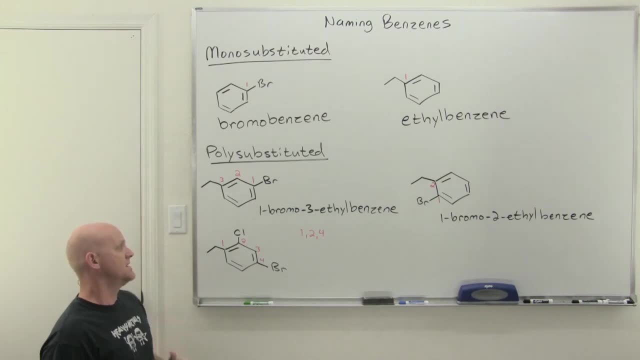 is one superior way of numbering. this Didn't have to use the alphabet to break the tie at all. We will still name these in alphabetical order, though, And so in this case we'll start off with bromo in the alphabet. So we'll say four bromo, and then chloro is next in the alphabet. So 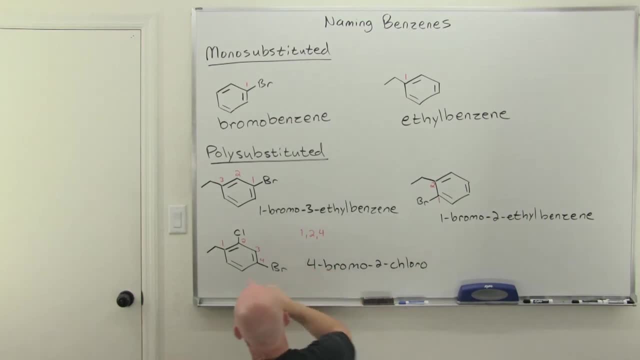 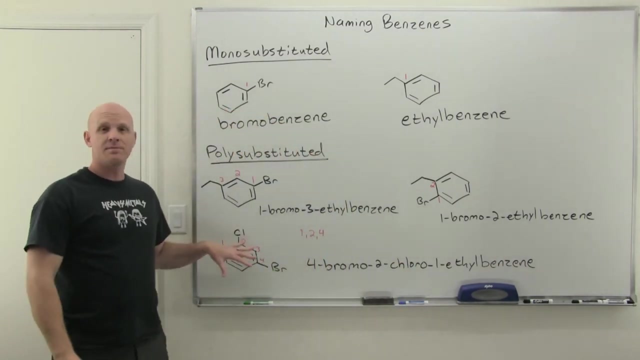 two chloro, one ethyl and then benzene. Cool, And I just want to cover an example where we had a tri-substitute or something more than that, because, again, a lot of students want to try and choose where number one is located. on benzene, 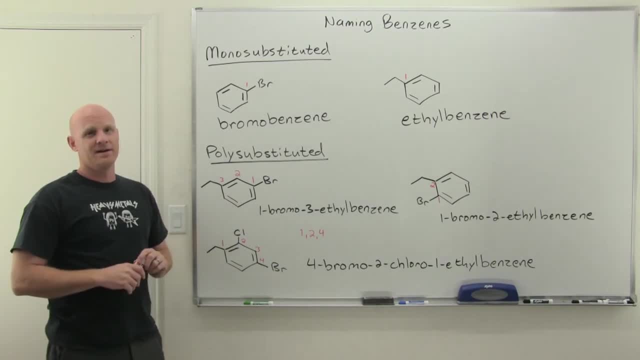 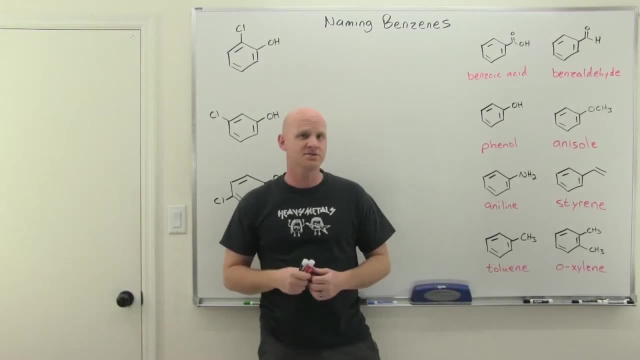 using the alphabet in such a case, And it usually doesn't come down to that. All right, let's go through some more examples here with benzenes with special names. All right, So now we're going to take a look at naming benzenes with some special names And. 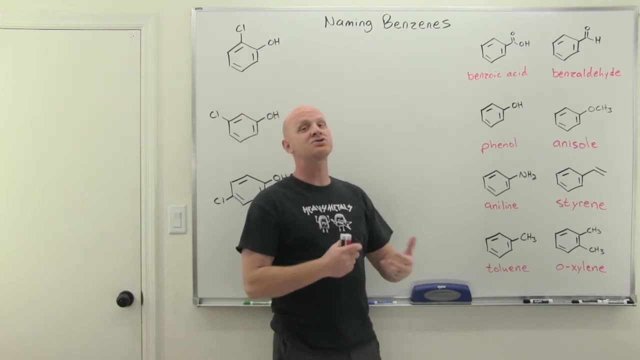 it turns out there are certain substituents. when they're attached to a benzene, they get a special name. So first one here is a carboxylic acid. So if you were going to name this with a very systematic IUPAC name, it would actually be called benzene carboxylic acid, And we'll learn. 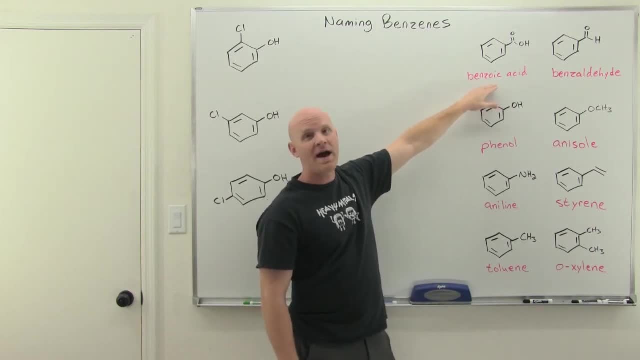 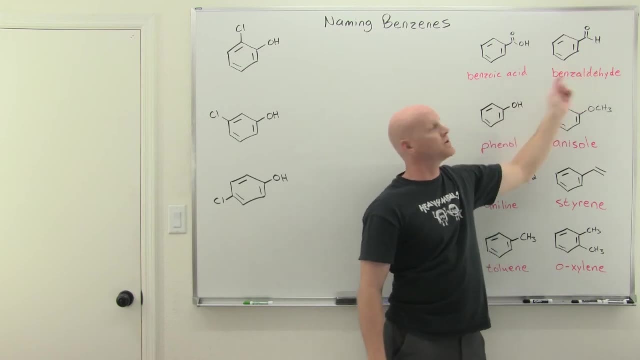 carboxylic acid. in the future, However, though, the IUPAC common name that is also accepted and much more commonly used is benzoic acid. Same thing here when you attach an aldehyde group to your benzene. Again the IUPAC name for naming an aldehyde. 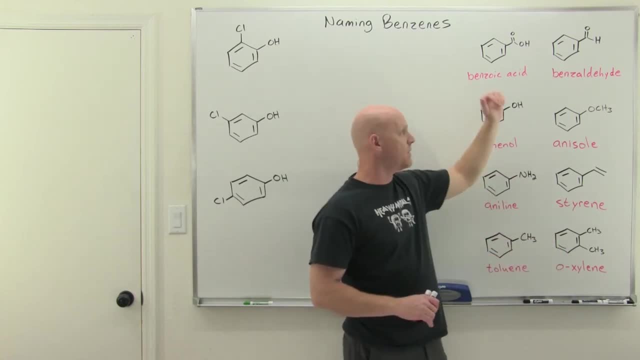 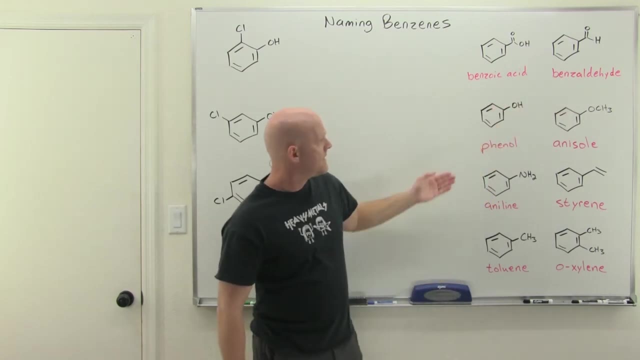 like this would be benzene carbaldehyde. So, but again, almost nobody uses that name. you'll much more commonly see it as benzaldehyde, And that common name again, is one accepted by IUPAC. All right, so when you've got benzene with a hydroxyl group, we'll call that a phenol. 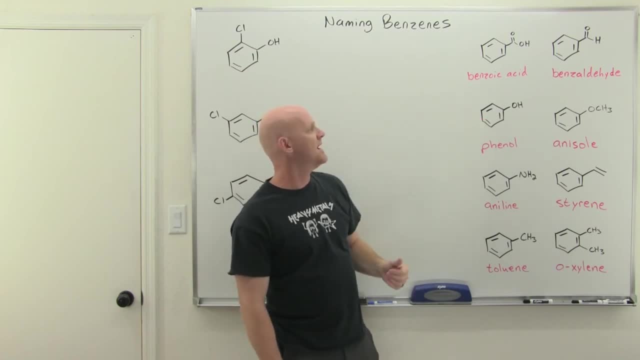 So that is not just a phenol. this is phenol the name, But in general we call them phenols. We learned about those back in the alcohol chapter. and methoxybenzene- here it's common name, much more commonly used as anisole for historical reasons. Aminobenzene again. 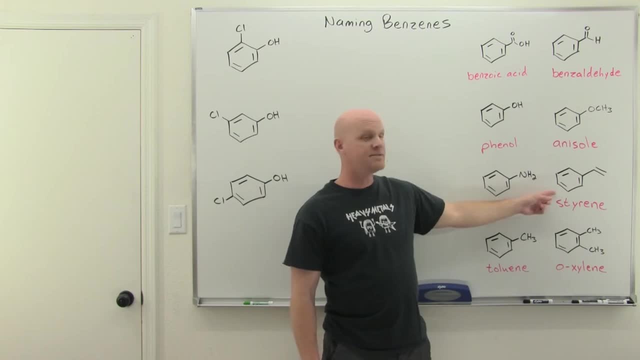 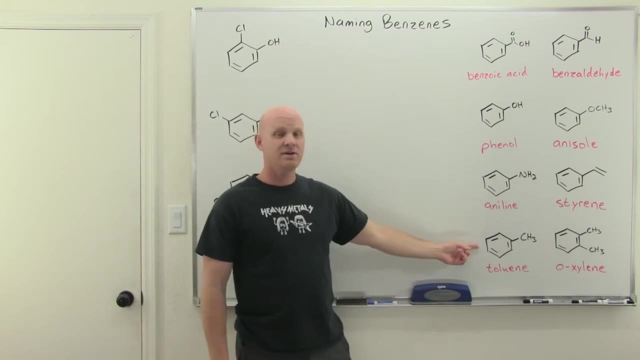 commonly called aniline. This here is styrene, vinyl benzene And styrene of. like polystyrene is actually a polymer made using styrene as the monomer. Here's toluene methylbenzene, much more commonly called toluene. This is: you put three nitro groups on there and you got. 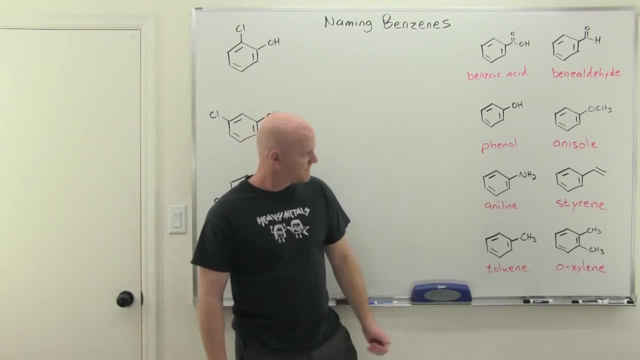 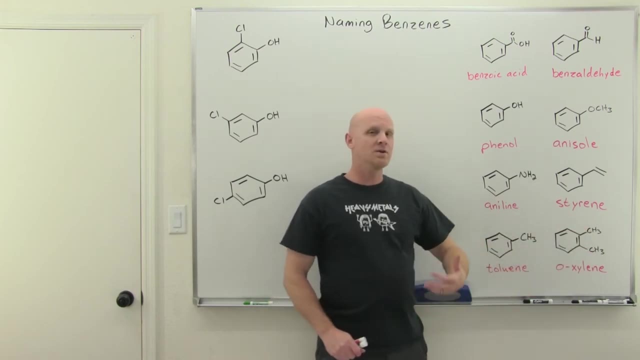 trinitrotoluene, aka TNT. So there's his fame. And then if you've got dimethylbenzene, it turns out that's going to be called xylene, And the two methyl groups can be oriented in ways and we'll kind of see the difference of what's going on there. All right, so those are. 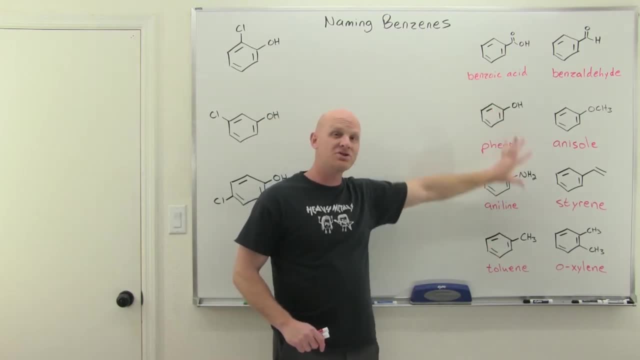 your special ones. And when you name a benzene with one of these special names, then the substituent that it kind of identifies will be identified as being at carbon number one of the benzene. So you know, if you name something as a phenol, so then as the parent name anyways. 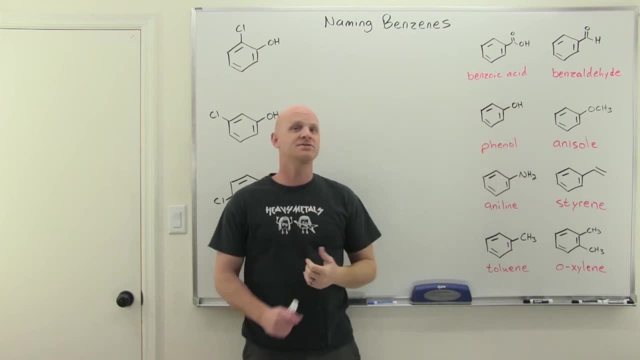 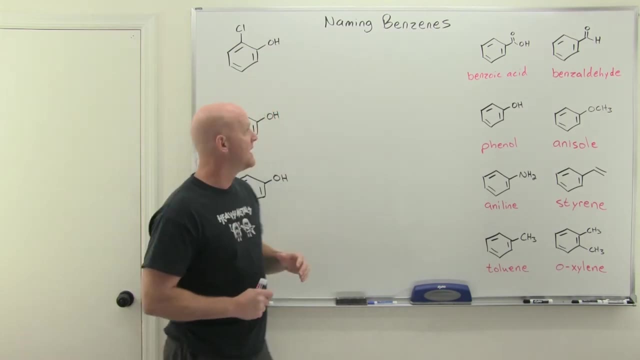 then the number one on the benzene will be right where the OH is attached by default. That's kind of how that works, So let's take a look. So we're going to start with some disubstituted benzene that we call phenol, And in this case we'll see a little bit different. Instead of using the 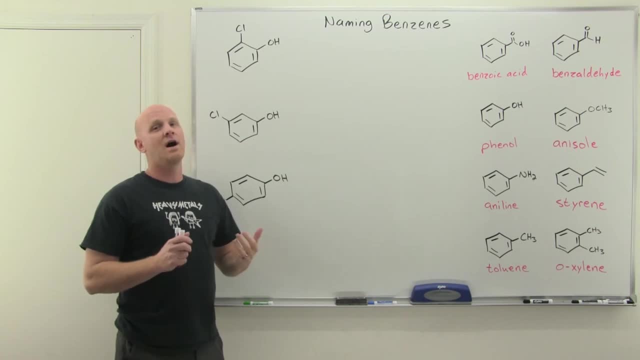 numbering system which you can still use. there's nothing wrong with that. We also have one other option. So in this case, notice, there's no special name for the chlorine. That's just chlorobenzene, if you have, you know, a chlorine on a benzene. But there is a special name associated with the OH. 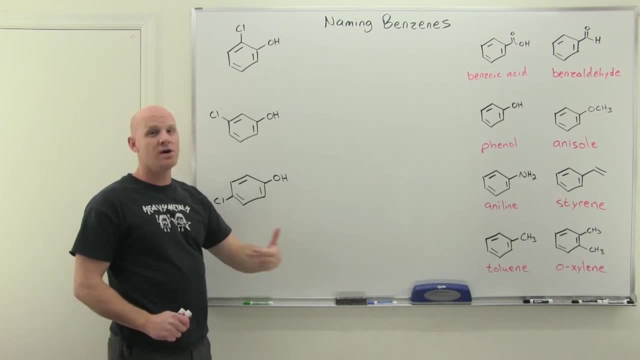 And so most of the time, you'd more commonly see this named as a phenol rather than like hydroxybenzene, And so in this case, if we call it phenol, though, then that automatically makes this carbon number one of the benzene. So and then to get the lowest possible. 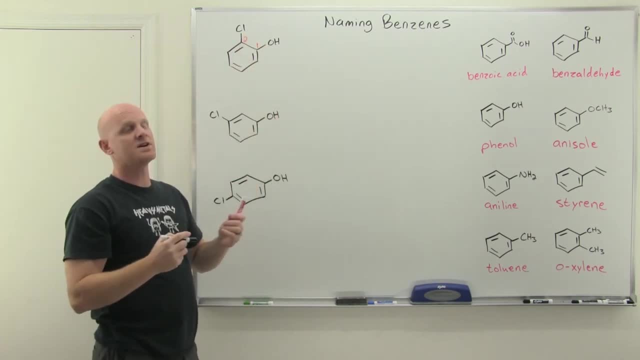 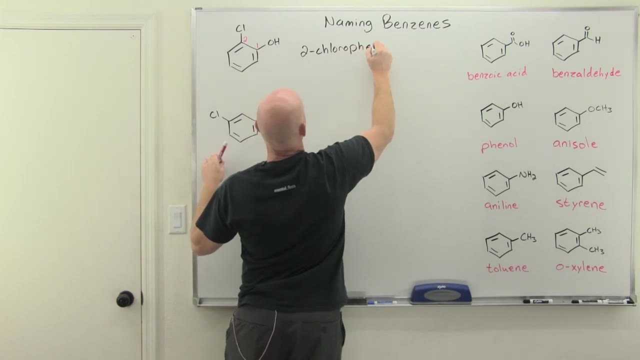 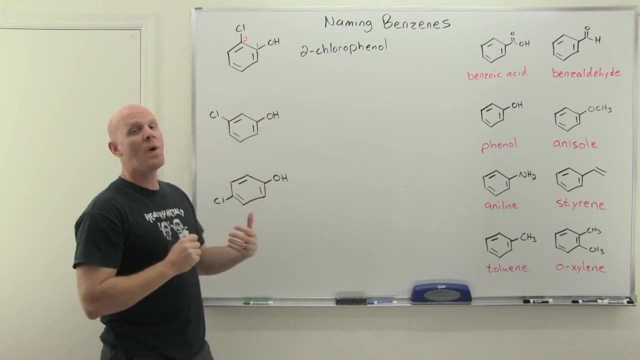 number. this would then be carbon number two, where the chlorine is attached, And so we've got a couple of different options here. We could call this 2-chlorophenol, or it turns out with disubstituted benzenes. when you have a special name, you have another option to identify where. 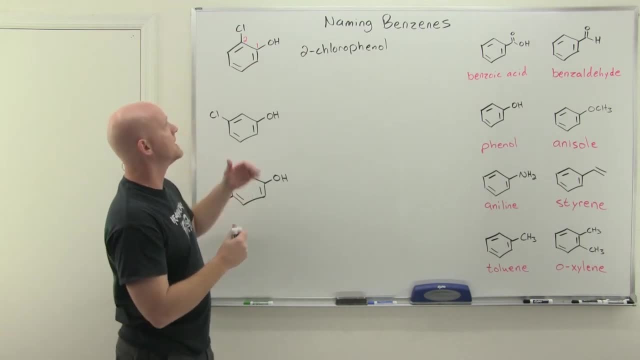 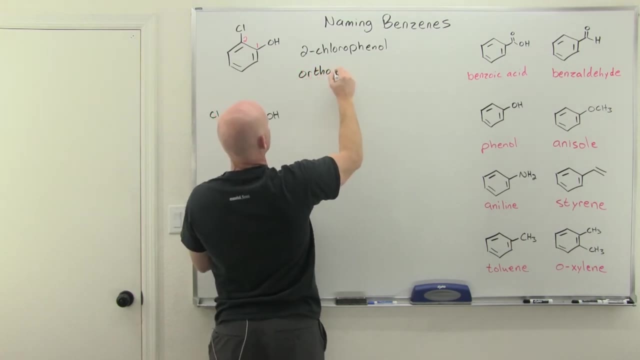 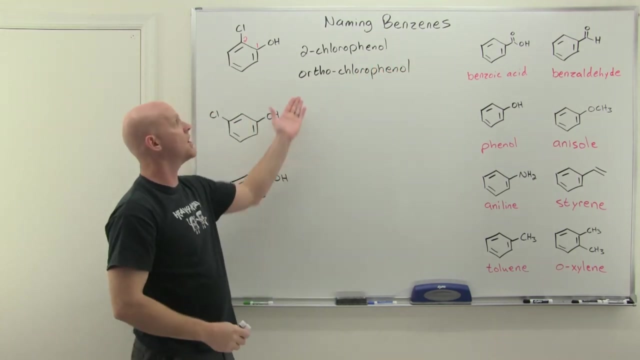 is that second substituent relative to the parent chain's functional group, And in this case for the 1-2 relationship. we call that ortho, And so you could call this ortho chlorophenol as well, And sometimes we just shorten it to O-chlorophenol, just like we did. 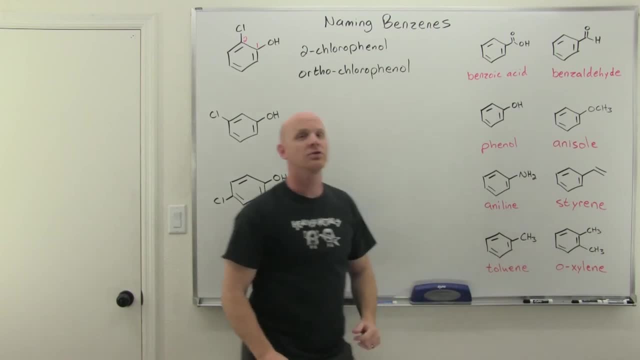 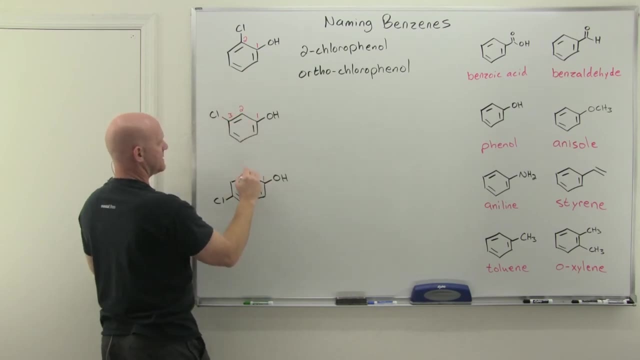 O-xylene down here, when the two methyl groups are in that 1-2 relationship. That's the first one, So we've also got here, in this case, a 1-3 relationship, And then here, regardless of whether I go clockwise or counterclockwise on this one, it's gonna be a 1-4 relationship. 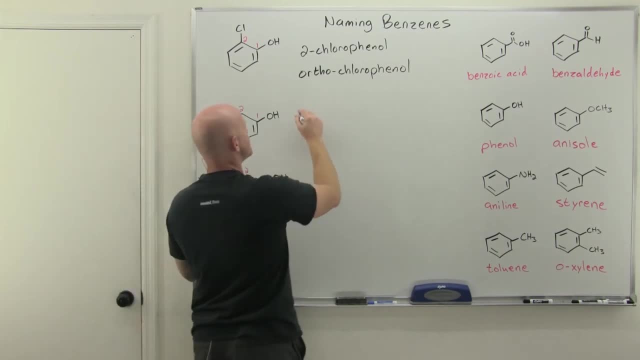 And those have special names as well. But again, you can still use the numbers, There's nothing wrong with that, And so you could call this 1-3. Chlorophenol, So, but it turns out you can also call it metachlorophenol for this numeric. 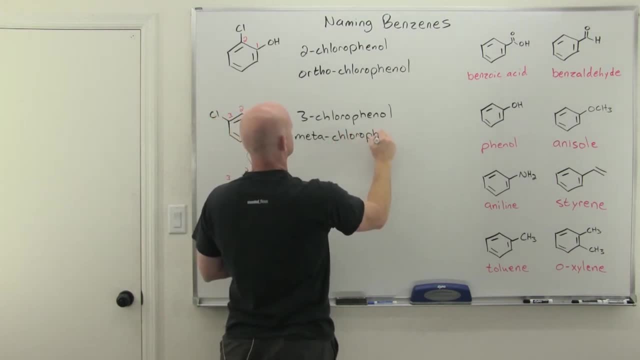 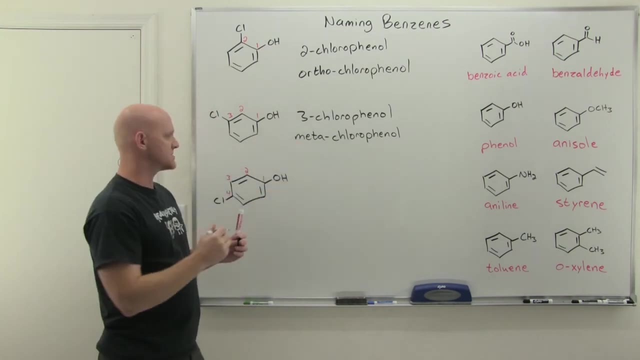 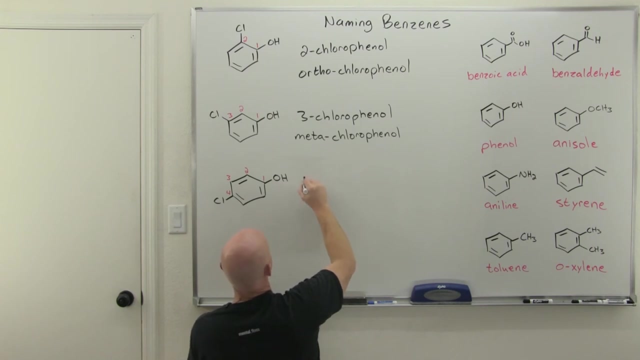 relationship, And sometimes we'll just shorten this down to M little little case, M chlorophenol. So totally acceptable as well. Same thing on this last one here. Now with the 1-4 relationship, it turns out we call that para So, but again you can still use the numbers. This is 4. 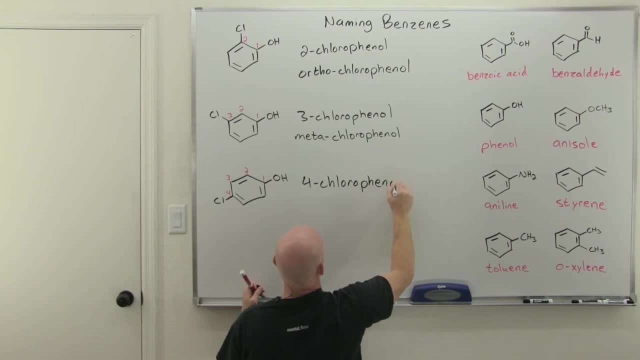 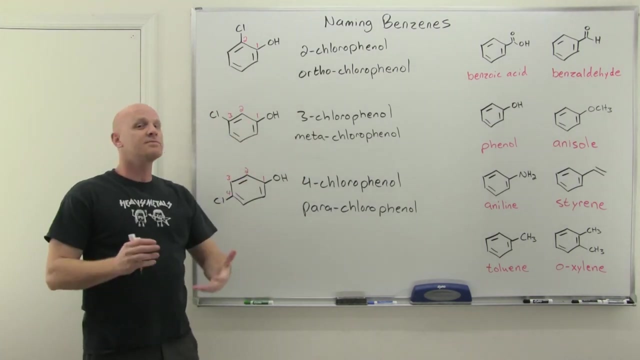 chlorophenol, But you could also call it para Chlorophenol or simply P chlorophenol for short. Cool, So for disubstituted benzenes. instead of the numbers, you'll actually much more commonly see ortho. 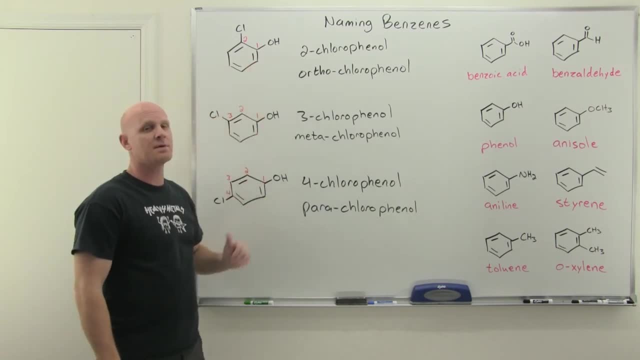 meta and para used. So, but these are also going to be special terms when we talk about reactions in the next chapter. So, because it turns out that when you've got a reaction involving a benzene, certain positions on the benzene might be activated or deactivated. 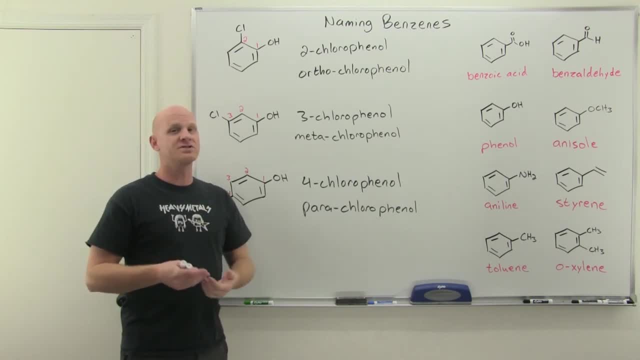 So you'll hardly ever see anybody identify with the ortho, meta and para relationships instead of, like the 2,, 3, or 4 relationships. You'll hardly ever see anybody identify it in such fashion. So, really important, you understand what ortho, meta and para mean and understand. 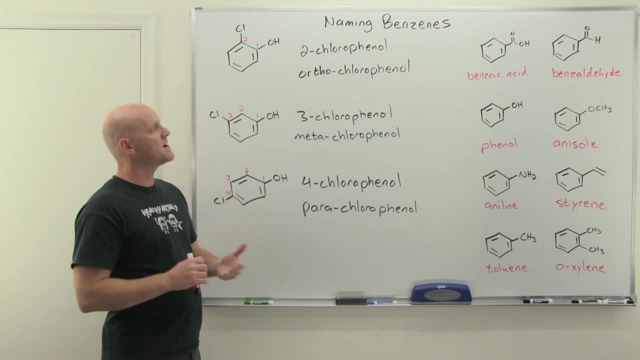 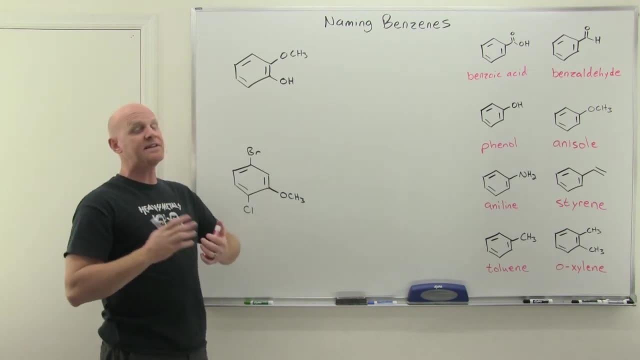 how they can be applied to nomenclature here with disubstituted benzenes when you've got one of these special benzenes involved. So I want to take a look at a couple more examples of benzenes with special names, And in this first one here we actually have two different groups that both 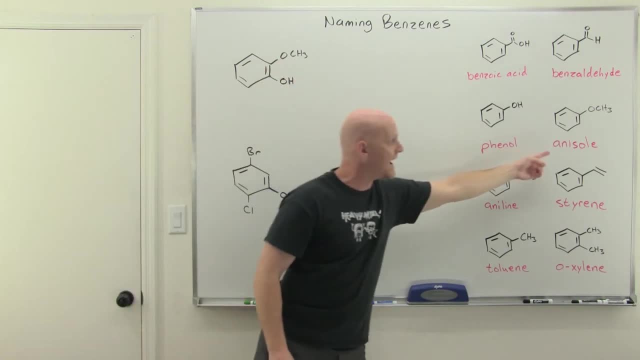 have a special name. So we're going to take a look at a couple more examples of benzenes with them associated with them. So methoxybenzene is also called anisole And again, hydroxybenzene is. 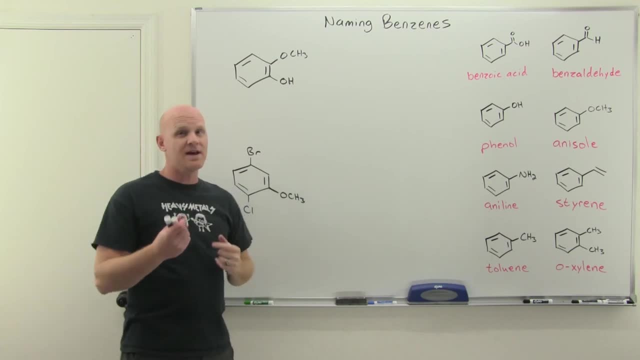 also called phenol, And so you actually get two different ways you can name this. So if we name it as a phenol, then automatically again that becomes carbon number one, which means where the methoxy group is located would be carbon number two, And so you could name this: 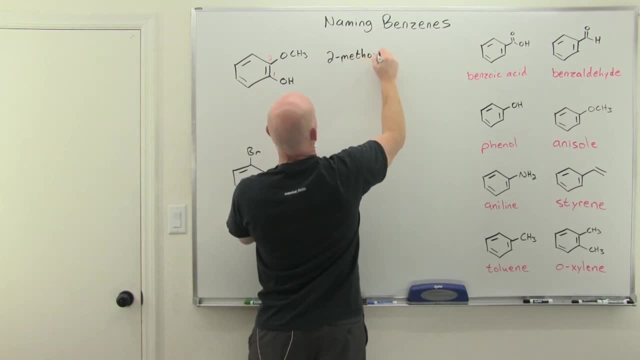 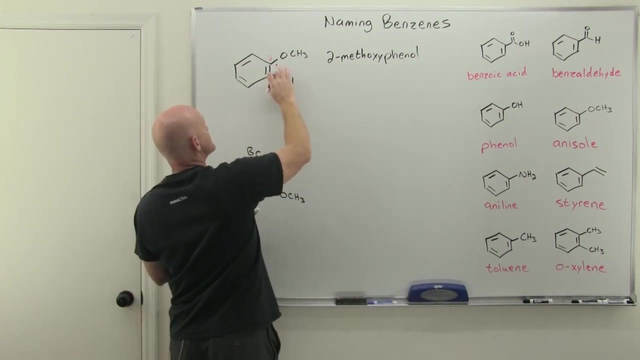 as 2-methoxyphenol. but we could have chosen to name the methoxy group as part of the major special name, So we can call it anisole, So that'd be carbon number one And the hydroxy group. 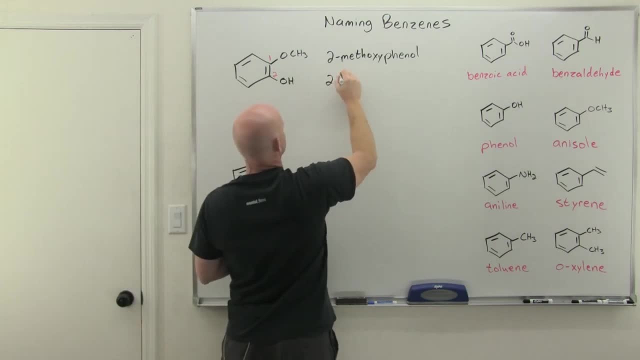 would be carbon number two, And so in this case we now call it 2-hydroxyanisole. Cool, And both are totally acceptable. So commonly, if you look this up, you'll see both names associated with. 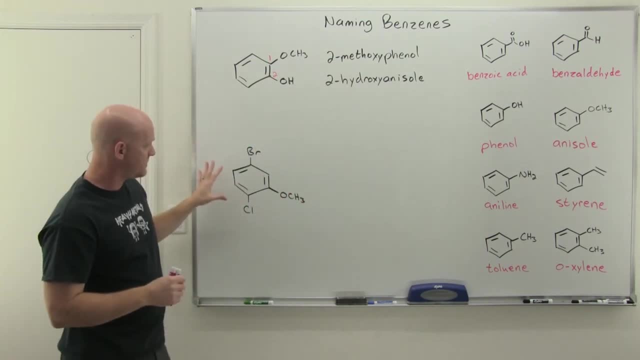 this lovely compound, both accepted by IUPAC, All right. So what if we go up here to a little more substituted benzene, And this is going to be 2-hydroxybenzene, So we're going to call it 2-hydroxybenzene. 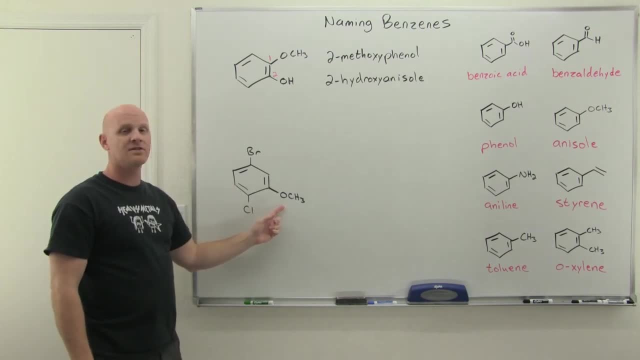 So in this case we've got a bromo, a chloro and a methoxy, and only the methoxy gets a special name, And so most commonly then you'd see us choosing that to be carbon number one We call. 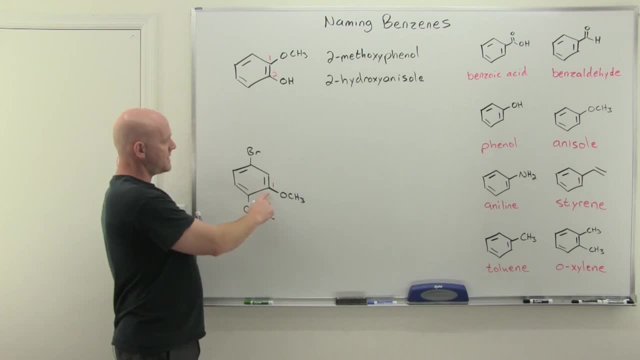 this anisole, again for methoxybenzene, And if we make him number one because we're going to call it an anisole, well then the lowest number I can get. the next substitution when I come across is if: 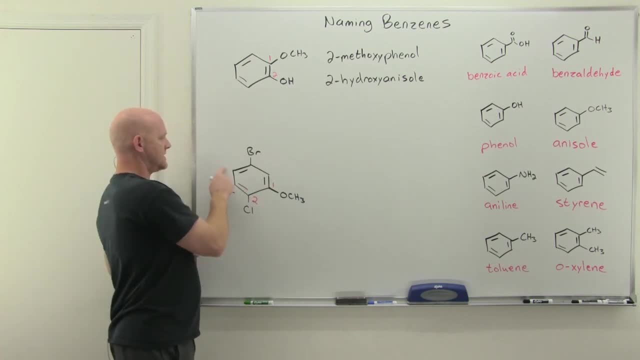 I number this clockwise and put the chlorine at two, and then keep going and put the bromine at five. So in this case we've got bromo-chloro-anisole, and we'll name those as 2-hydroxybenzene. And so we've got a bromo-chloro-anisole, and we'll name those. 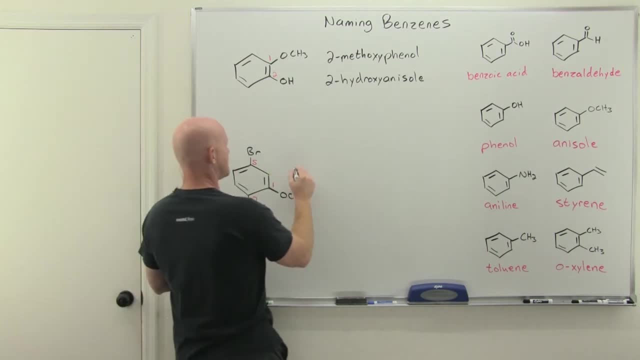 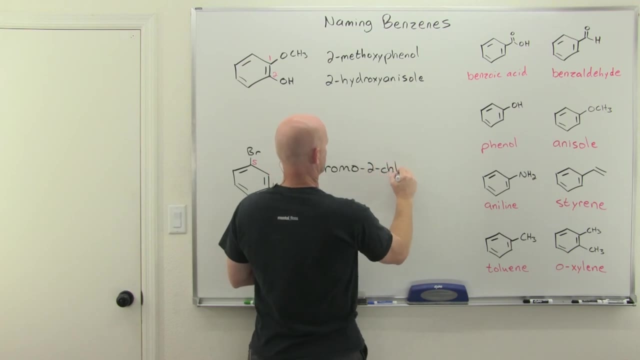 the bromo and the chloro in alphabetical order. So we'll start with that bromo, And so we've got 5-bromo and then 2-chloro and then anisole for the parent name. Cool, That's kind of how that. 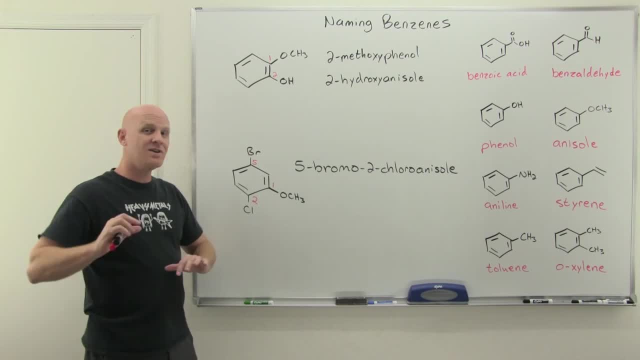 works And once again, you could try and go through this and not use anisole as the name and just have like methoxy and chloro and bromo and stuff like this, And that's where things get a little bit confusing and you're less commonly going to see that. So if you've got one of these, 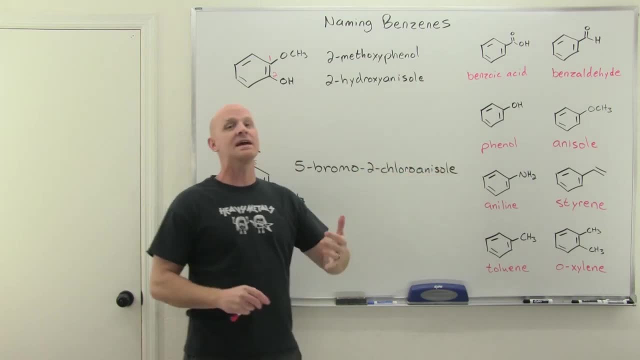 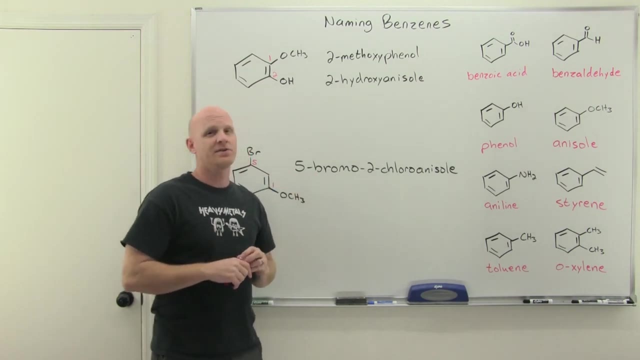 special benzenes, you are way more likely to name your benzene as special benzene Or, if it's presented to you, you're way more likely to be given the name with one of these special names incorporated.